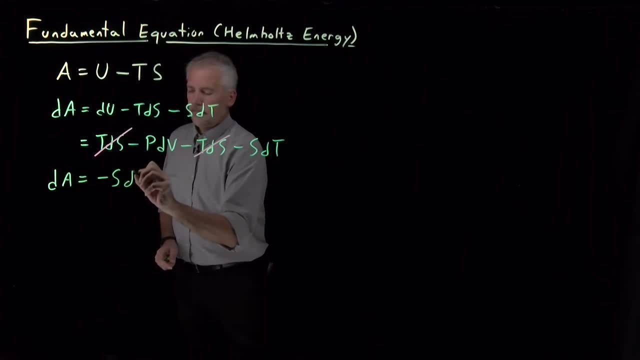 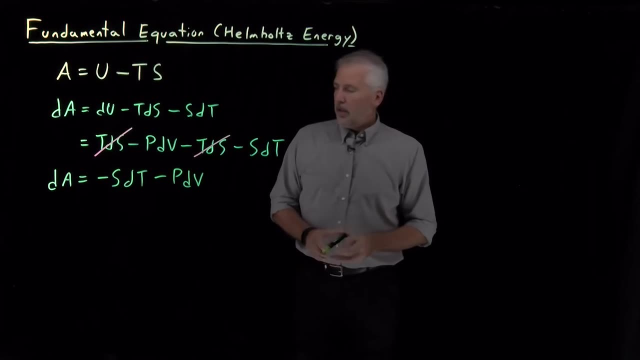 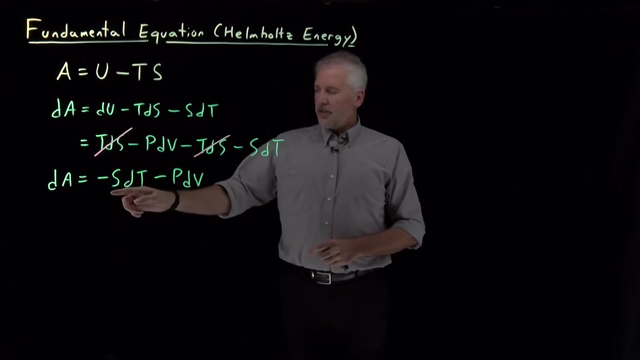 order of these two negative SDT minus PDV. So very similar to this. These are the fundamental equations we've seen before for the internal energy and for the enthalpy. The difference here is in which differentials- the differential of A- is expressed in terms of. 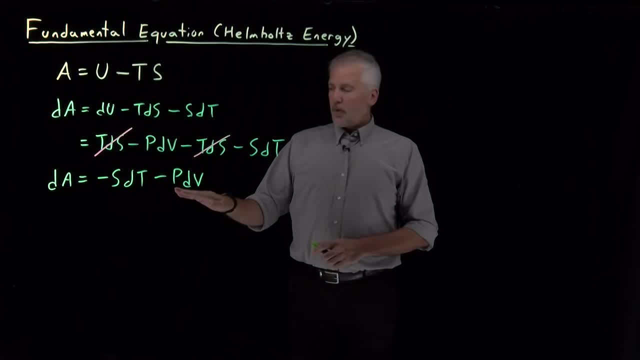 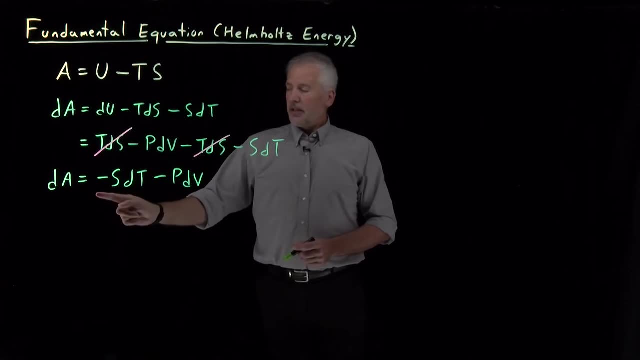 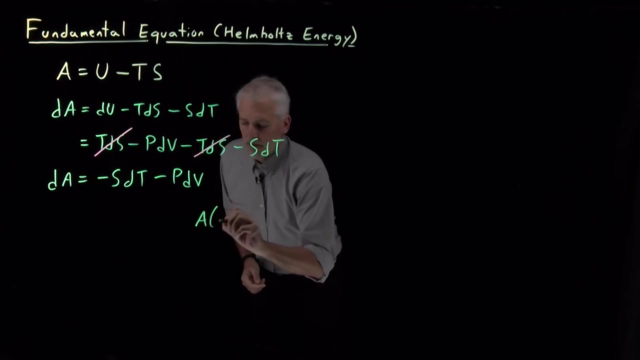 And this tells us immediately several things. One, it tells us that the natural variables of the Helmholtz energy are T and V, because this DA has this nice, clean and simple form when expressed as a function of DT and DV. What that means is that if we think of A as a function of DT, we're 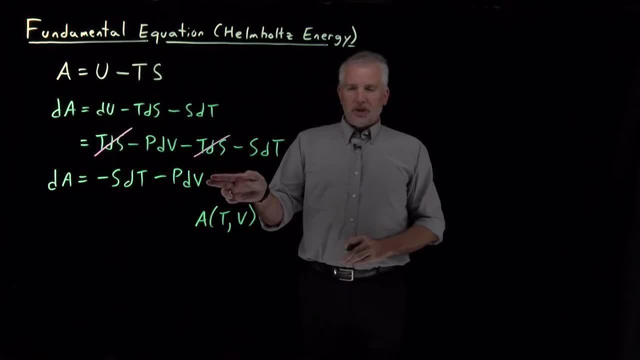 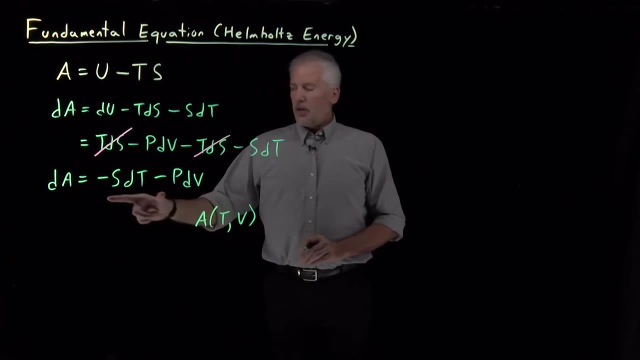 going to think of A as a function of T and V. This expression is simple. If we were to think of A as a function of T and P or S and P, or S and T or some other combination of variables, we could obtain a. 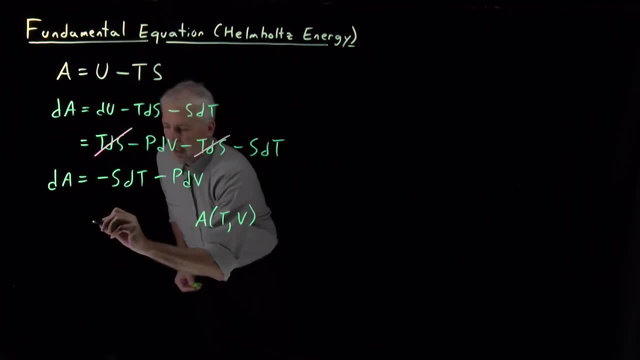 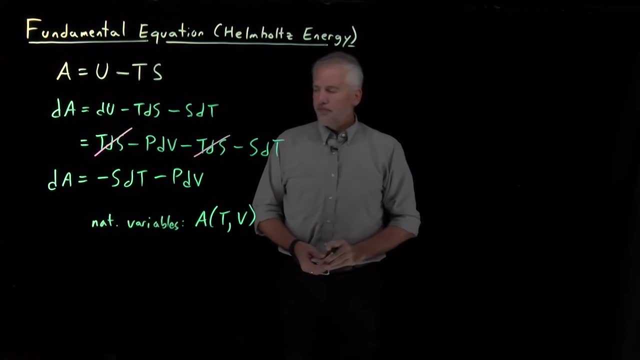 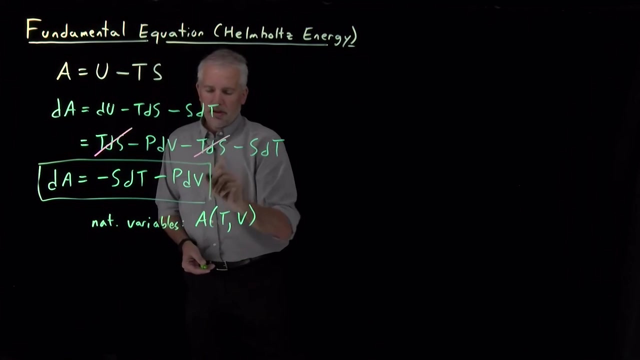 differential, but it wouldn't be quite as simple. So natural variables for Helmholtz energy are temperature and volume, The other thing we can see immediately from this fundamental equation. so I'll put the fundamental equation in a box, because that's when we'll come back to. 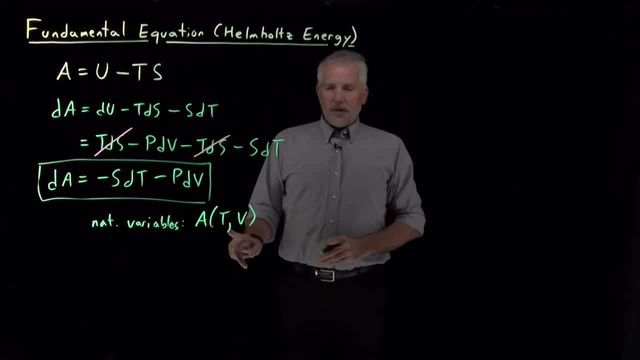 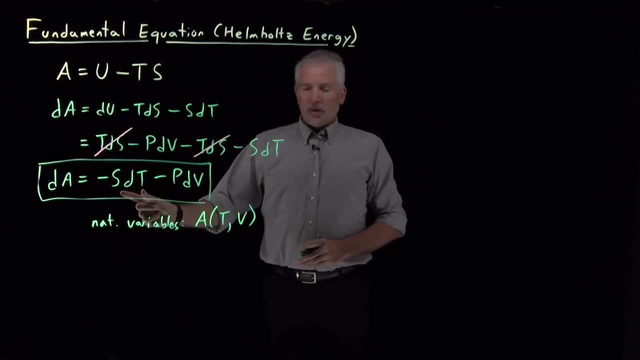 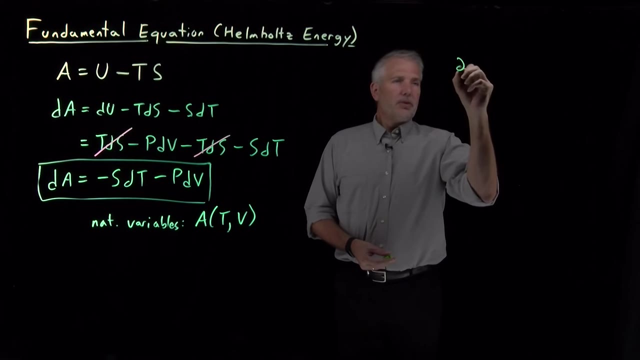 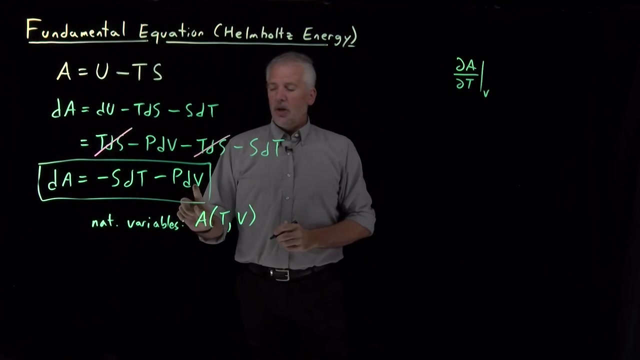 over and over thinking of A as a function of T and V, writing DA as some change multiplied by some coefficient multiplied by DT and some coefficient multiplied by a DV. this term, negative S, is equal to the rate at which A changes when we change the temperature. DA, DT when V is held constant. So we 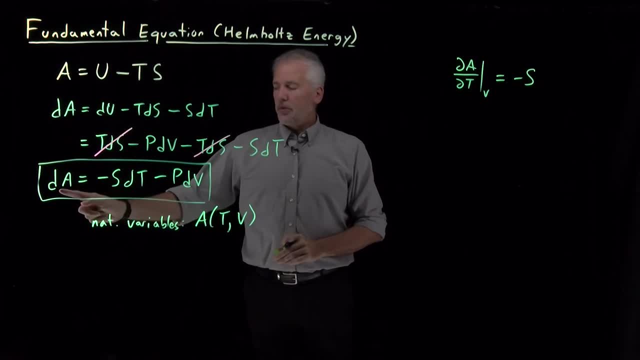 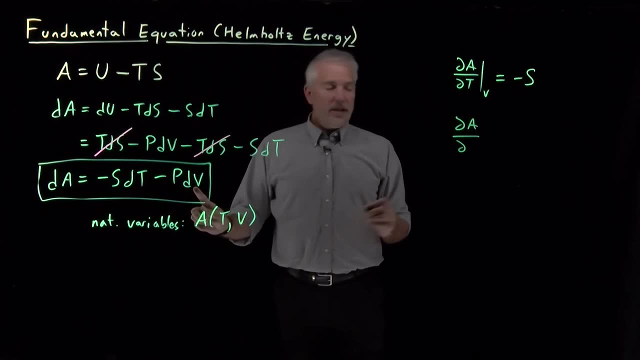 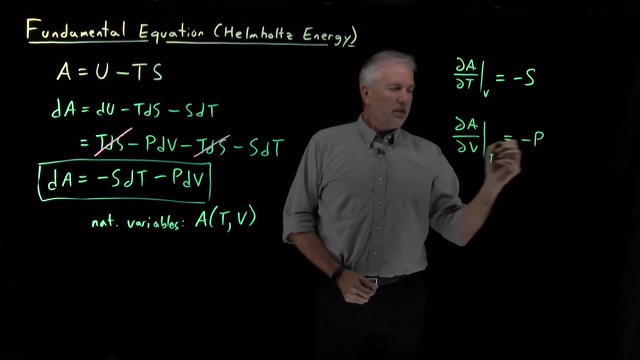 can read directly off of this fundamental equation. So negative S is equal to DA DT at constant V, and likewise DA DV, when T is held constant, is equal to this coefficient negative pressure. So those are useful expressions. We can add those to our toolbox of. 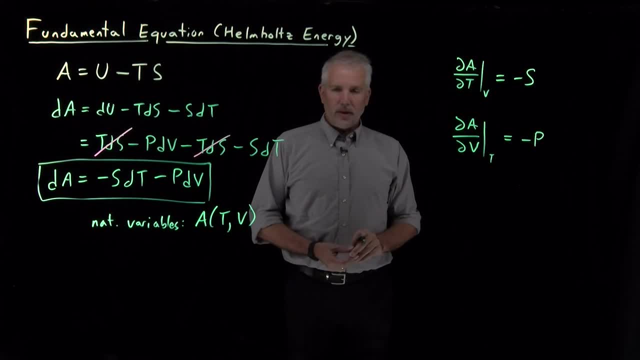 thermodynamic derivatives. That's a list that's growing quite steadily and we'll see more of them as we go forward. If we were ever to happen to want to know how quickly the Helmholtz free energy is changing as we change the temperature, as we change the volume, while holding the other one constant, these 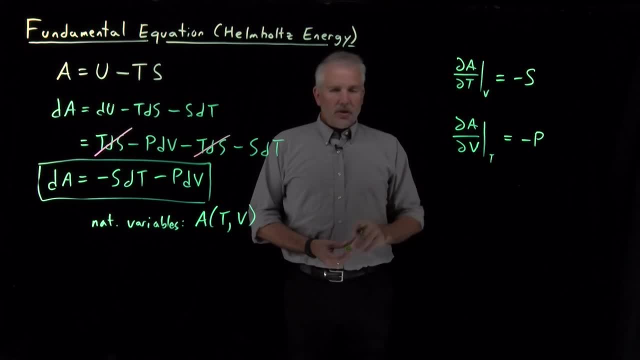 expressions tell us how to do that. So we'll make good use out of those expressions and others like them, but for now we'll move on, and the next thing we'll do is to obtain the thermodynamic connection formula for the Helmholtz free energy, while we're talking about the Helmholtz energy. 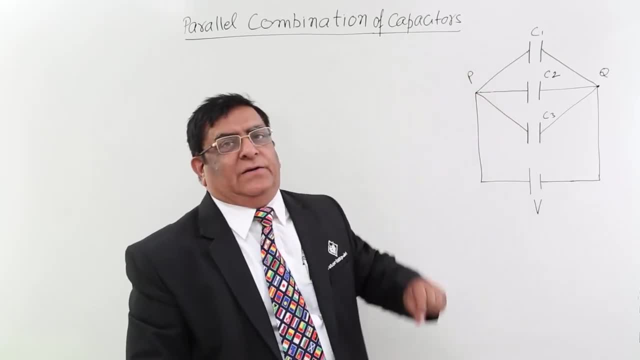 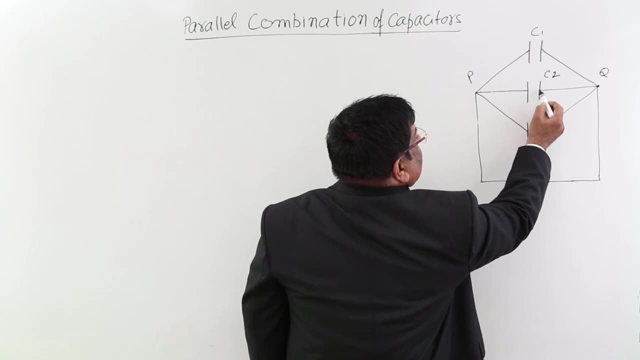 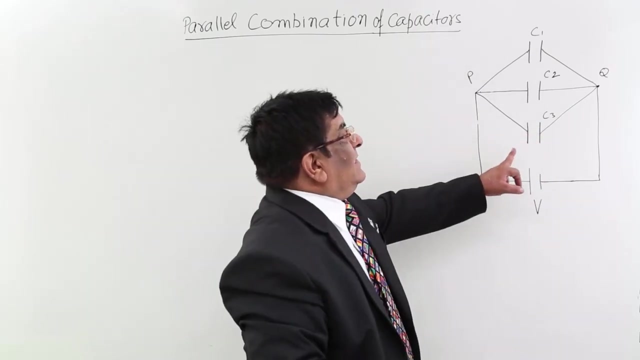 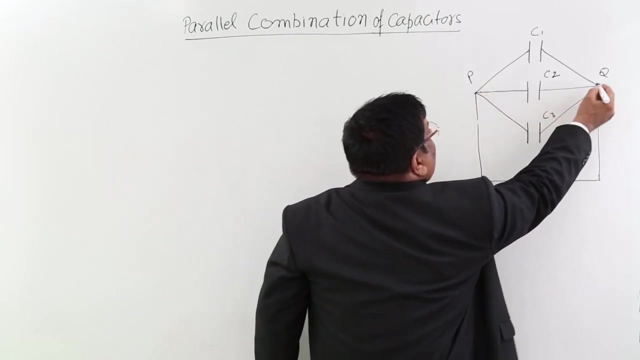 Now we will study how capacitors are connected in parallel. In this, first plate of each capacitor is connected, The other plate, second plate, is connected together. So these three will be known as in parallel. So these are combined in parallel. Now these are combined in parallel. 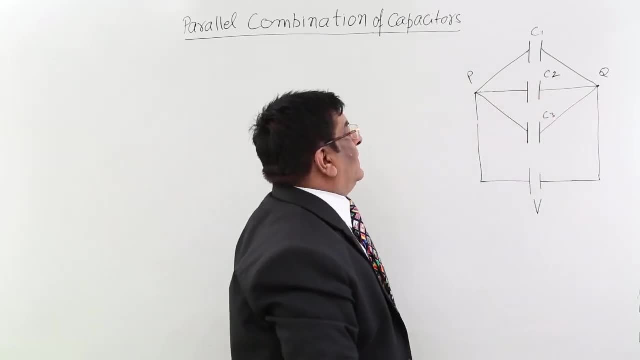 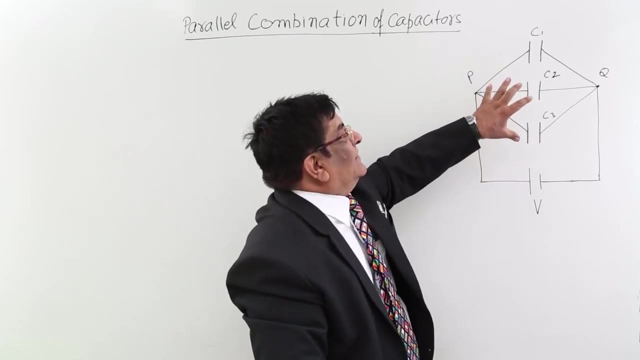 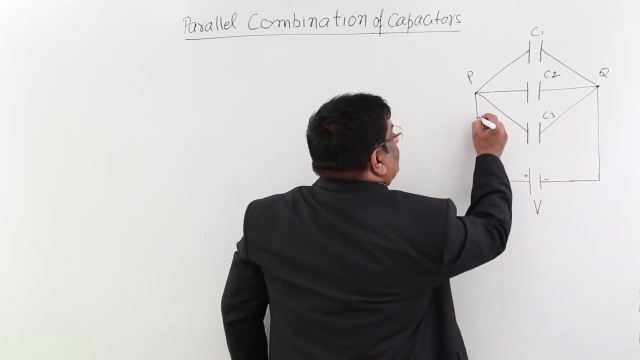 across these two points, P and Q. If these are between P and Q, this is a parallel combination. We want to charge it. If we want to charge it, we connect a battery across P and Q. From this, positive charges go up to P. This is one wire, But when they reach P they find: 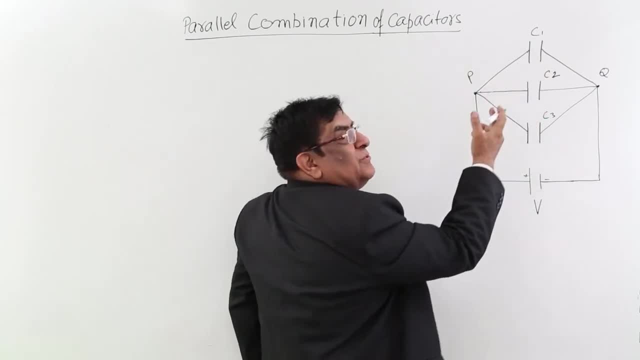 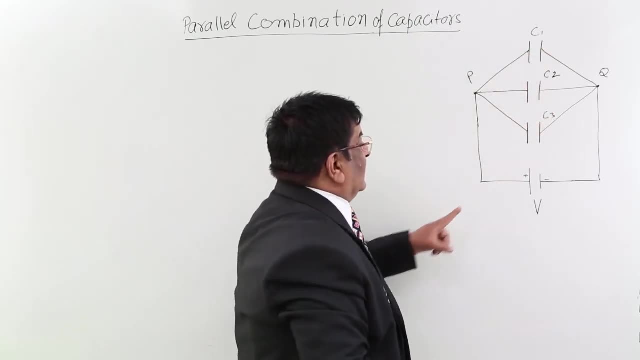 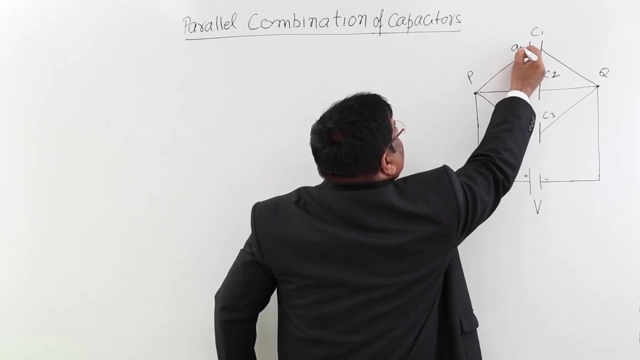 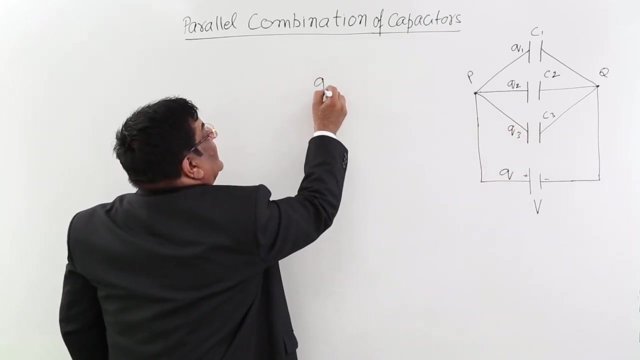 there are three paths And the charges distribute themselves in the three paths. Some charges go here, Some go here, Some go here. So if it has given total charge Q, Q is divided into 3.. This one gets charge Q1.. This gets Q2.. This gets Q3. And it is very obvious that the total 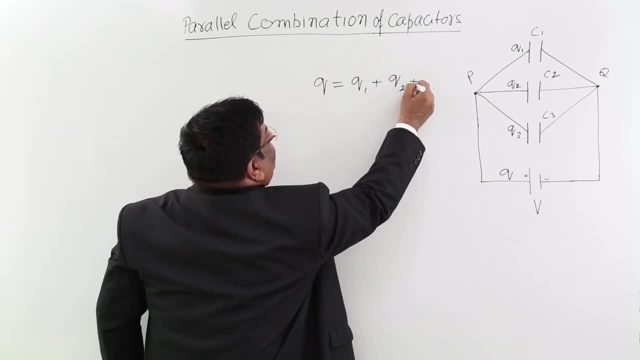 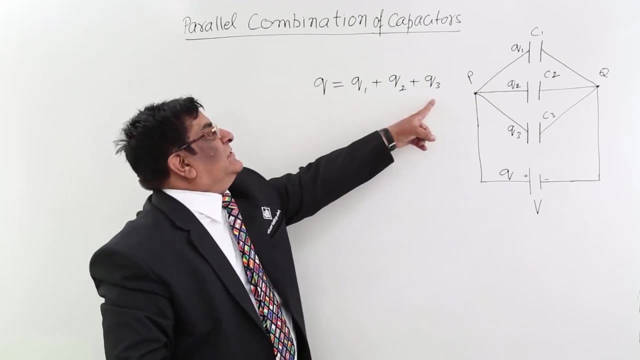 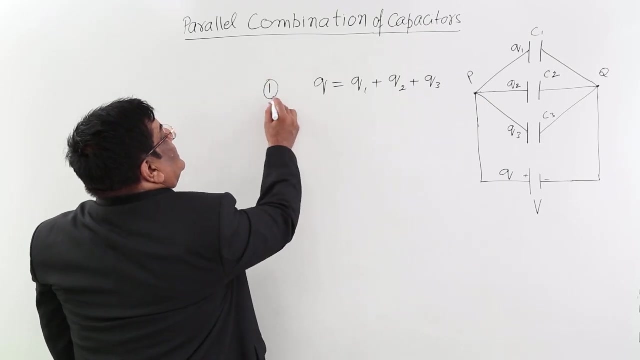 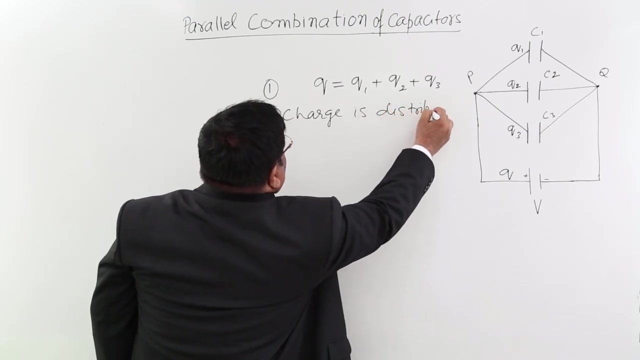 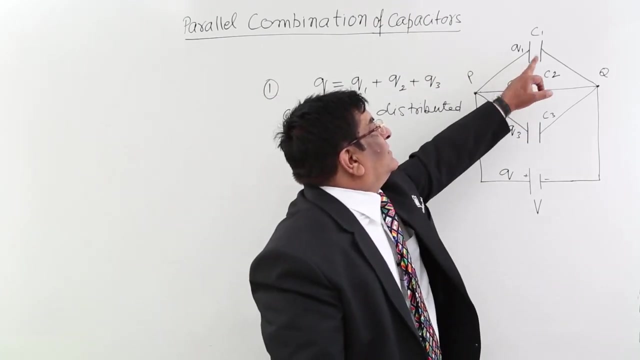 charges is divided into 3.. And this is something we cannot create or destroy, So the total charge has to come from Q. Physical charge is P and P2.. Physical charge is 0.. So because P and Q comes with these two paths or generation, Rom tu riju, these two Detailed charges and energy intensity. 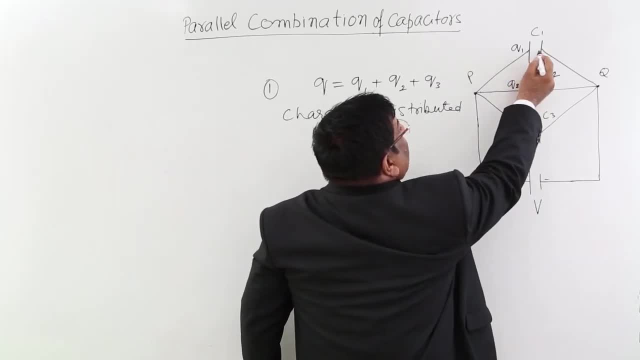 respectively. The power isшая. So this is the equation. total charge is Q1 plus Q2 plus Q3.. So first rule for charge: Charge is distributed. Now, because of this charge and its capacitance, there is some potential difference created here. this will do induction Because of its induction heat. some of these